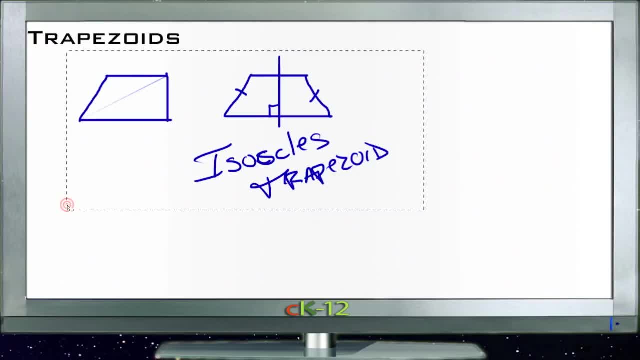 If it's not an isosceles trapezoid, all that really matters is that the top and the bottom are parallel to each other. Let's make a little bit bigger isosceles one here, so we can see what we're doing a little more easily. 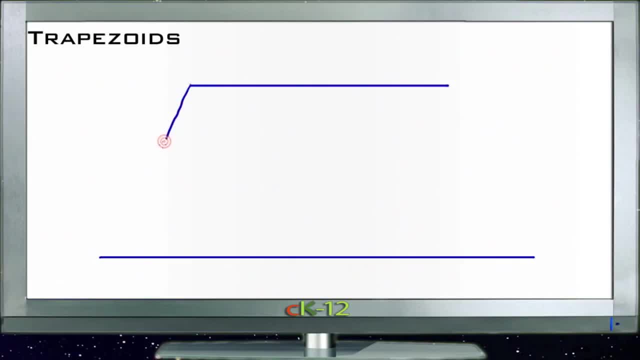 Here we go. Sorry, my diagonal lines are only kind of straight because I don't have a good straight line tool for those. There we go, We'll call these the same. Now that means if this is an isosceles trapezoid, then these angles down here, the base angles, will be congruent. 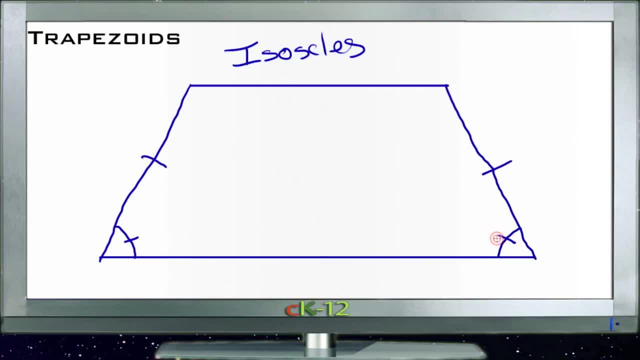 Right here. It also means that the mid-segments of both of these lines. if we were to connect the mid-segments of the two sides, then we have another line that is parallel to the top and the bottom and its length will be the average of the lengths of the top and bottom of the figure. 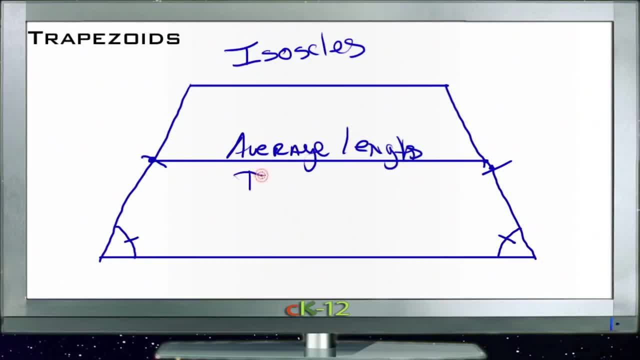 So, in other words, if we call this side A and this side B, then the mid-segment length would be A plus B divided by 2.. And that actually works for any trapezoid, but it's certainly much more apparent, I think, when you're looking at an isosceles trapezoid. 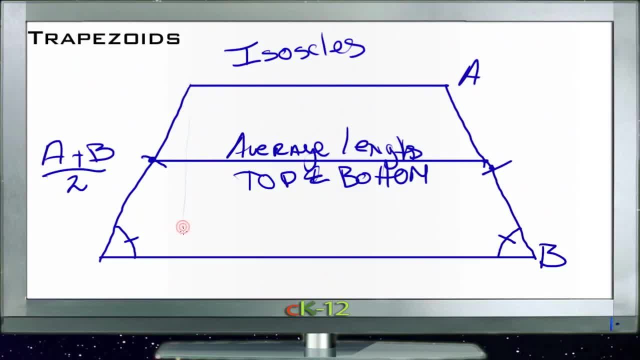 because basically, what we're doing is taking this line here, We're taking this distance here and here on both sides, and then we're splitting it so that we're taking part of it and adding it up here to effectively make the top and the bottom of the trapezoid equal like a rectangle. 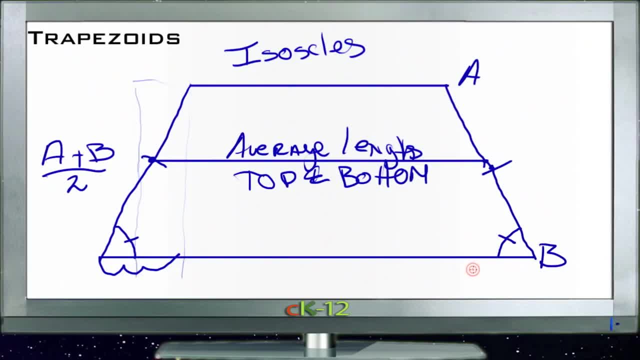 If you don't know that a trapezoid is isosceles and you're trying to prove that it is, you can either measure these angles down here. If the base angles are congruent, then this is an isosceles trapezoid. 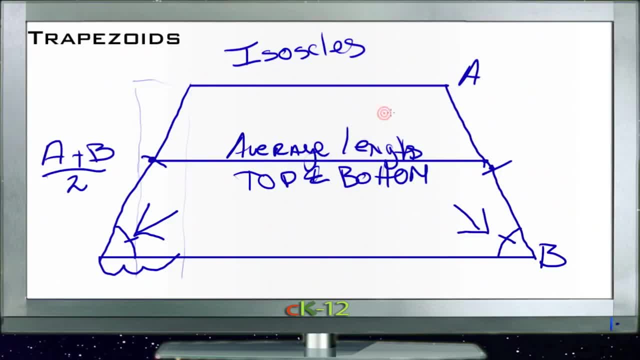 You can also measure the lengths of these lines here. We call this side here C and this side D. If C and D are identical in length and these two sides are parallel, this is either a parallelogram, which means that C and D are actually parallel to each other.